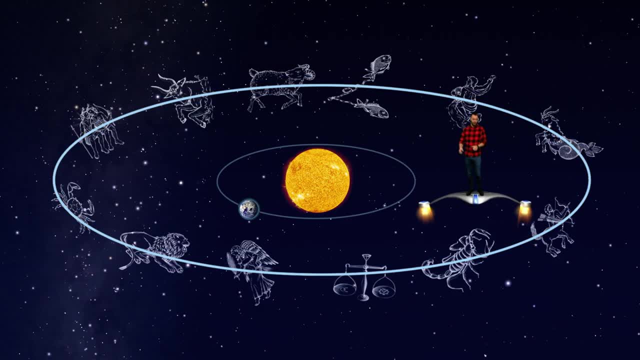 and around and around again. The tilt of the earth is what makes the sun swing up and down in the sky depending on the season, And that angle compared to the equator is called obliquity and it's generally 23.5 degrees. 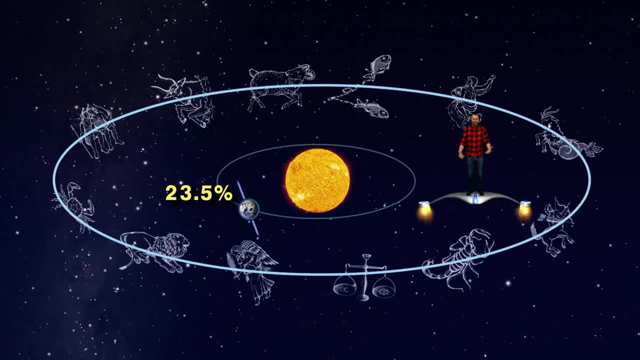 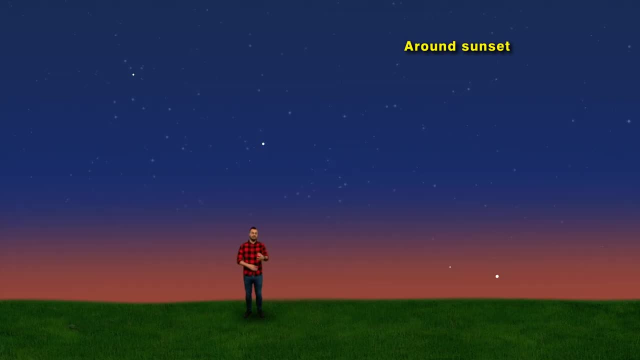 If the earth never wobbled, the sun would always follow the equator, Every day would be the same length. there wouldn't be any seasons. Sounds terribly boring. It's important to know the ecliptic because this astronomical pathway is where a lot of exciting stuff happens in the sky. 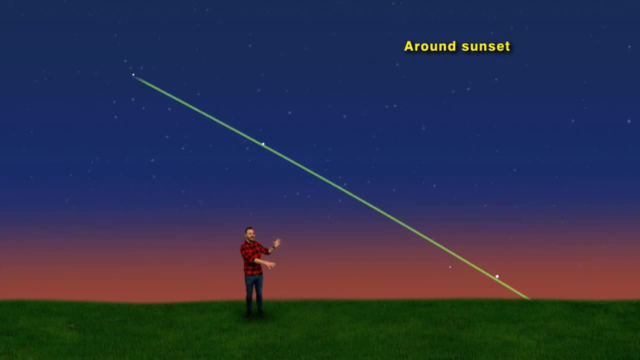 To find the ecliptic, go outside around sunset. If you trace a path from the sun through any visible planets, you'll notice that they form a line and this is the ecliptic. And it works because generally the solar system is pretty flat. 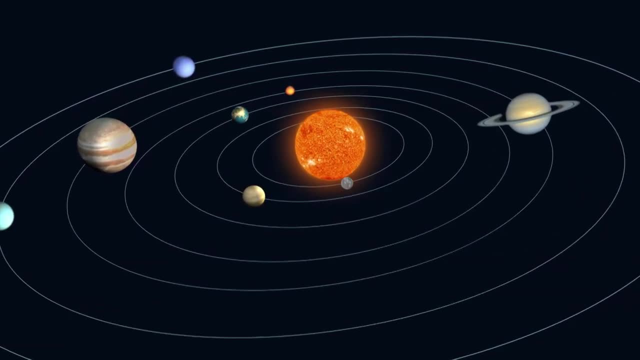 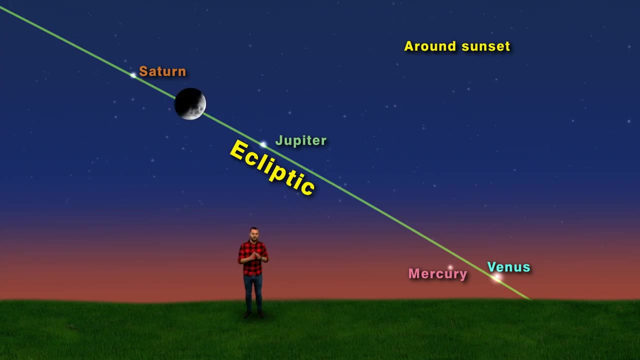 So all the planets follow a similar orbital plane, appearing either in front of or behind the sun as it plods its daily trail. Additionally, the moon is only a few degrees off from this plane, meaning if you know where the ecliptic is, you can predict where the sun and planets and moon will be on any day. 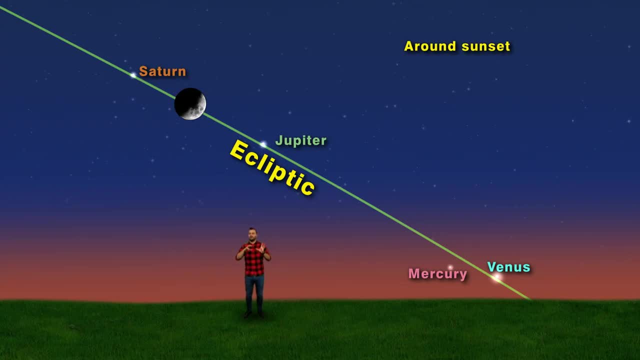 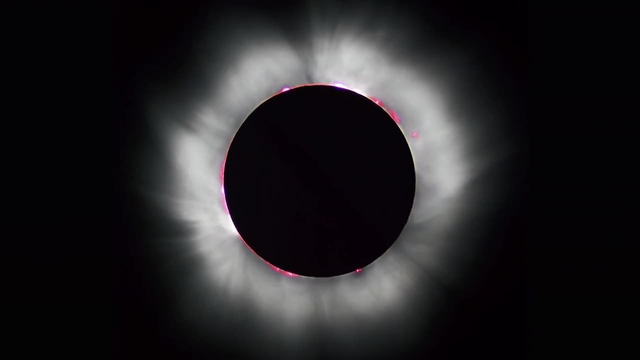 But that's not all. the moon's orbit is about 5 degrees off the ecliptic, and when things line up, that's when we get eclipses, Which is how the ecliptic got its name. When humanity first realized the sun was this predictable. 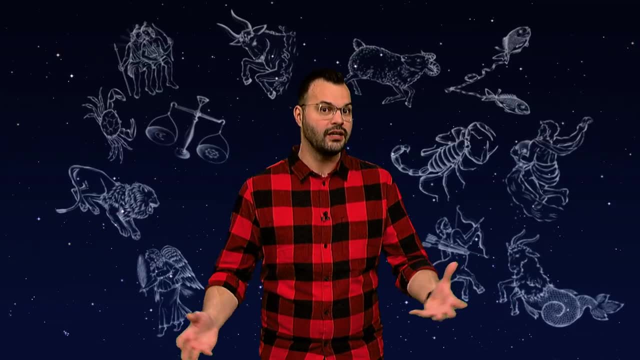 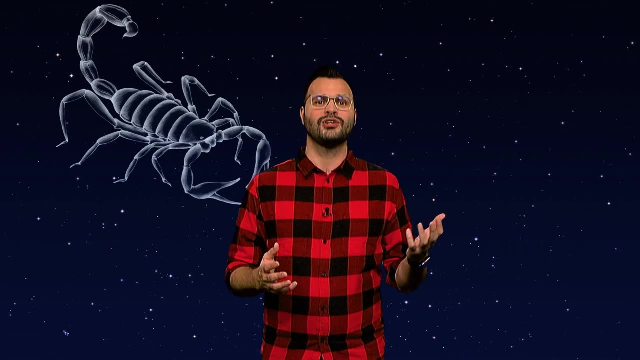 they found that it swept through each of the zodiac constellations yearly, Although over the last several centuries the tilt of the earth has shifted, meaning that the sun actually spends less than a week in Scorpio and nearly three in the 13th constellation, Ophiuchus. 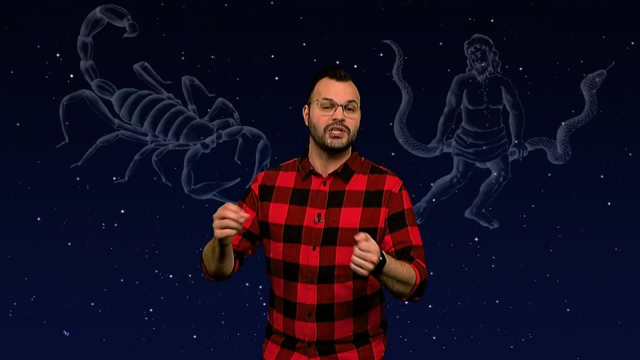 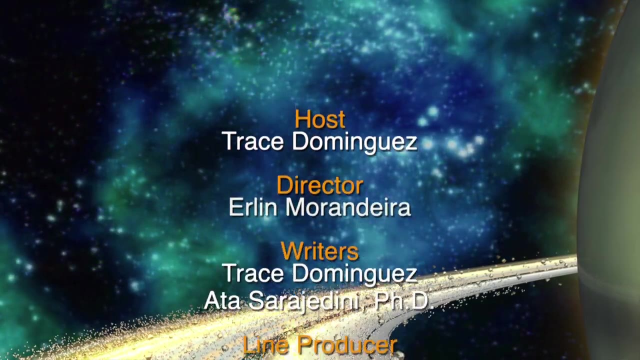 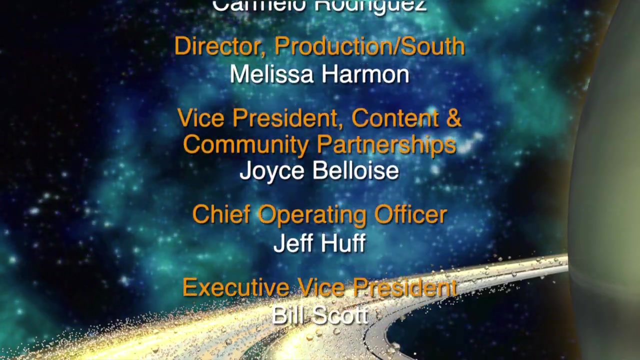 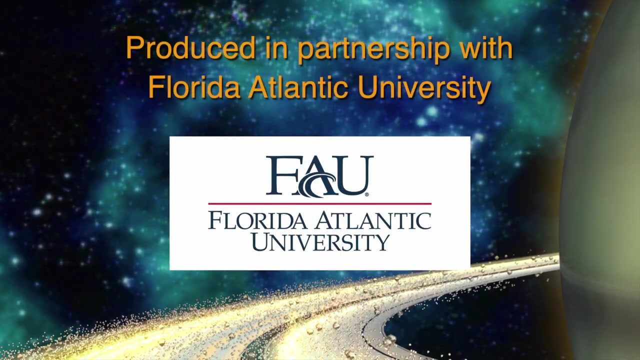 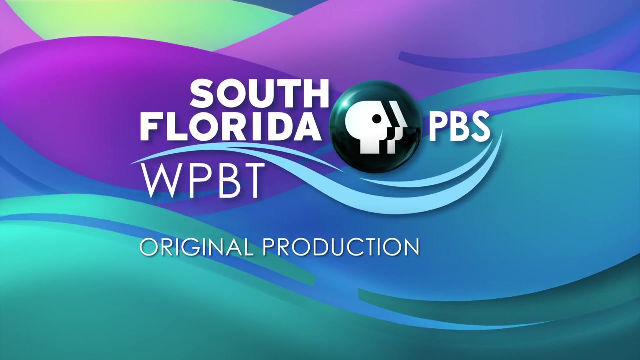 But hey, things change. Knowing the ecliptic will help you predict where things will be in the night sky while you keep looking up. Thanks for watching.